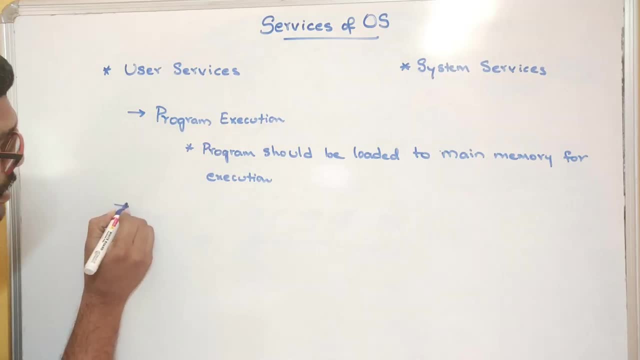 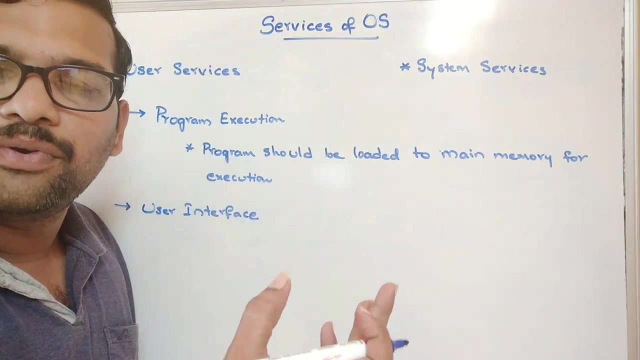 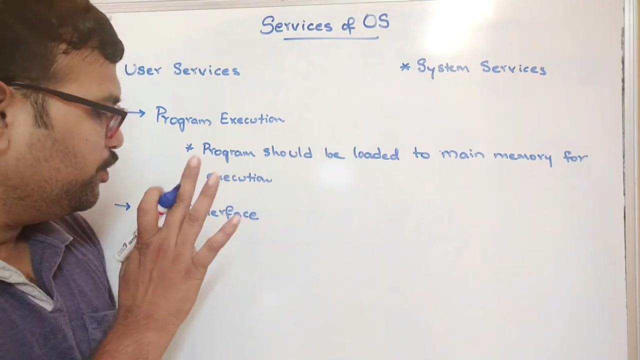 this operating system and the second service is user interface. so in order to communicate with the computer is somewhat difficult because the user have to communicate with the computer with the help of instructions. for everything you have to use some instructions and by using this interface it makes the easy. it makes the user very easy to communicate. 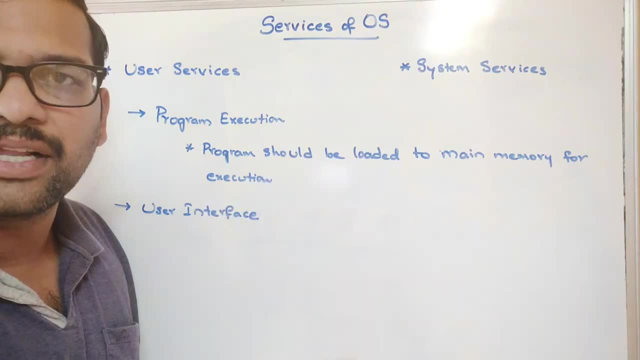 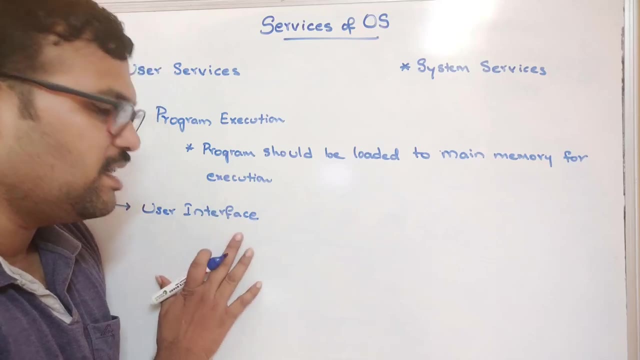 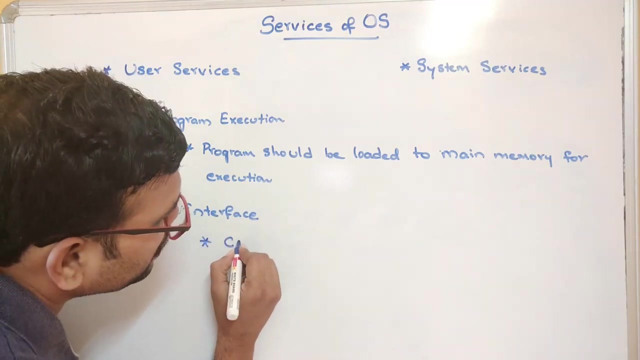 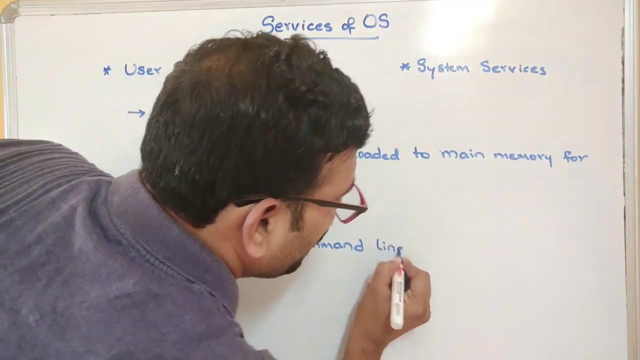 with the computer, right? so here the computer means the hardware, that means either processor or a memory or io devices, etc. etc. so the user can use this interface to easily communicate with the system. and this in interface is of two types. one is command line interface, cli, it's a command line interface, command line interface. so here. 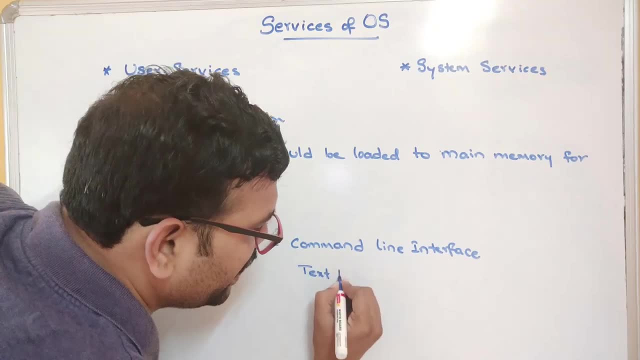 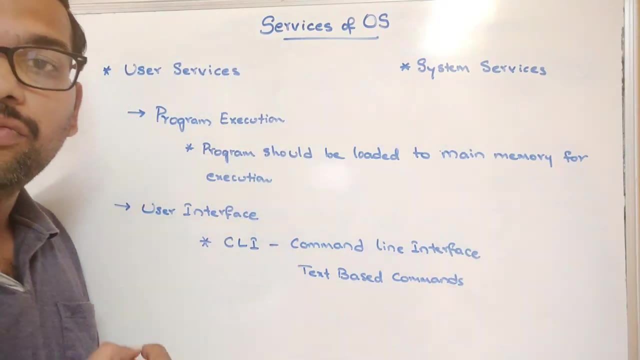 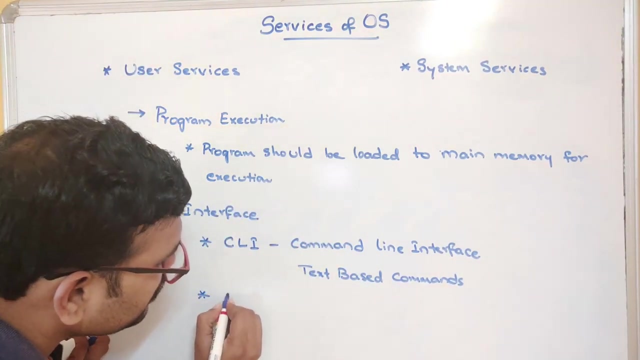 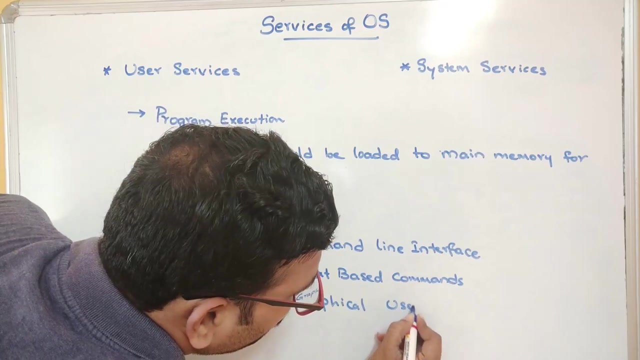 everything will be in terms of text based commands. text based commands- right, so the user have to give the text based commands in order to do the process. and there is a one more thing, that is a gui. gui stands for a graphical user interface, and this graphical user interface, this 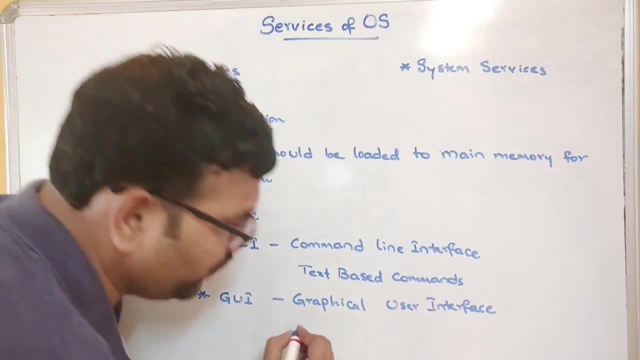 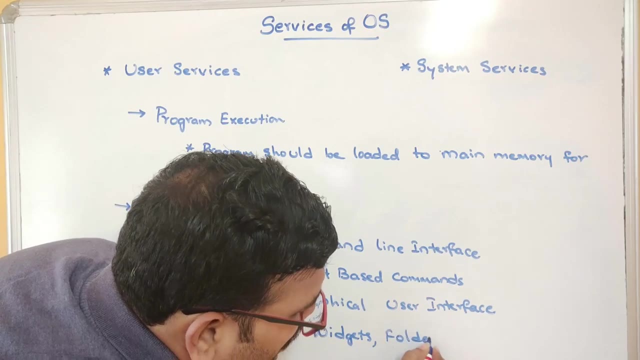 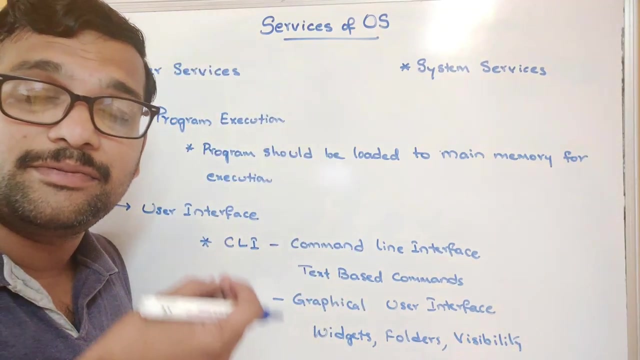 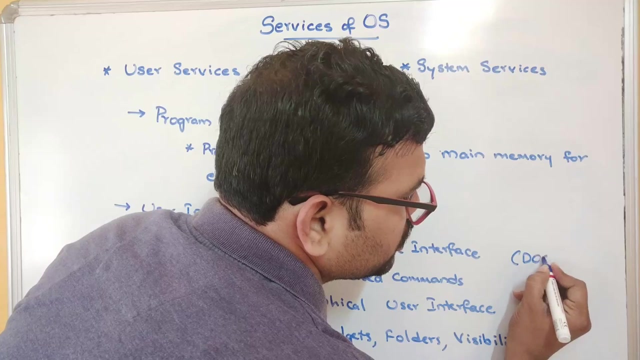 graphical user interface will be used by the user. that means we are having some widgets, okay, folders and some sort of visibility, right? so visibility will be more, visibility will be more, and this- this makes a user very easy to communicate with the computer, right? so example: we can go with the dos operating system, which is a command line. so for everything, even if you want to, 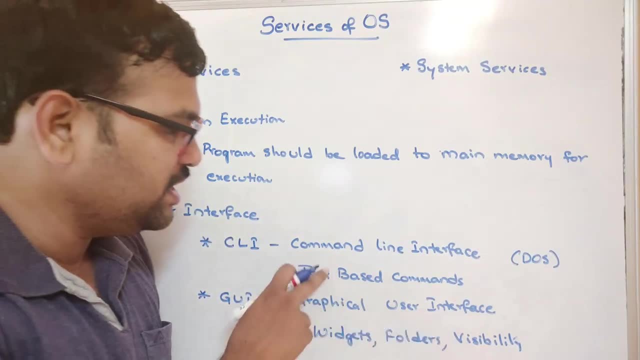 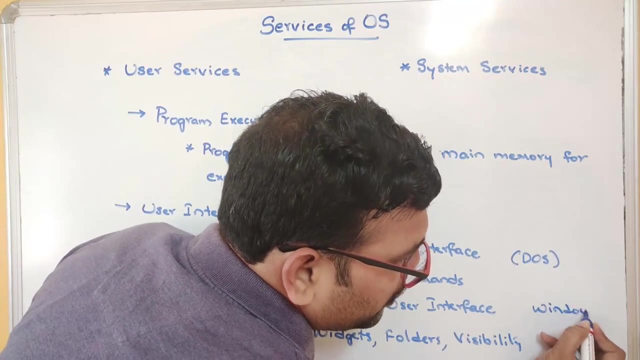 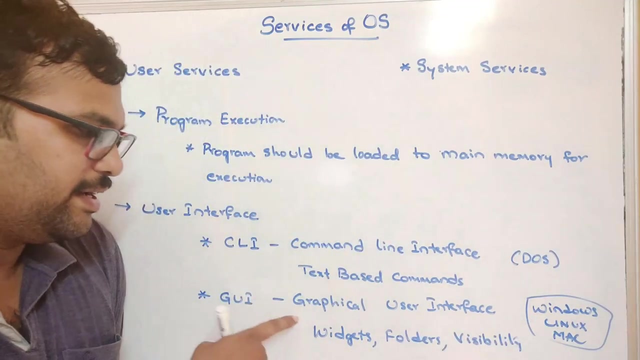 create a file. if you want to create a folder, we have to use this text-based commands in this particular operating system and graphical user interface. we can go with the windows, okay, linux, so mac, all these things. all these things comes under this graphical user interface, right? so we can create a folders or we can work on the folders of files. 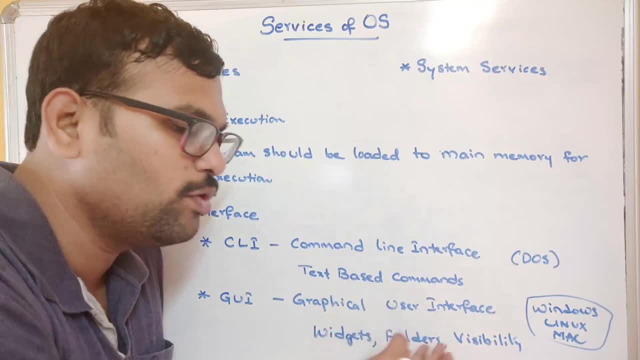 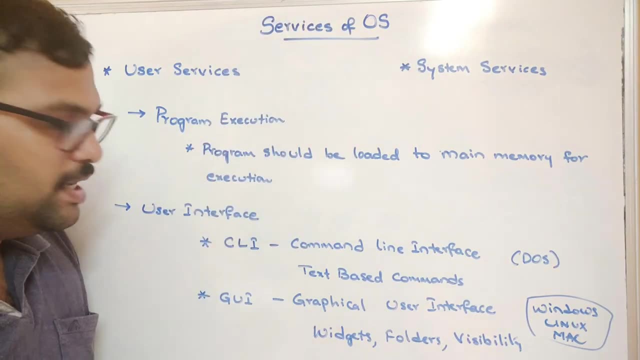 with a simple mouse moves and by using the widgets, folders, etc. etc. best feature provided by the operating system: right so, with this user interface, it makes the user very easy to interact with the computer right next. so I am discussing about this: user services. then we will go with the system. 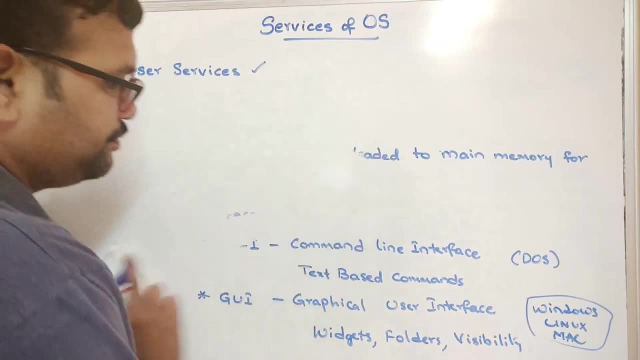 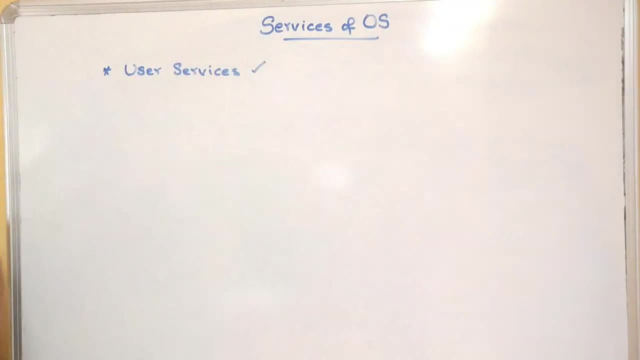 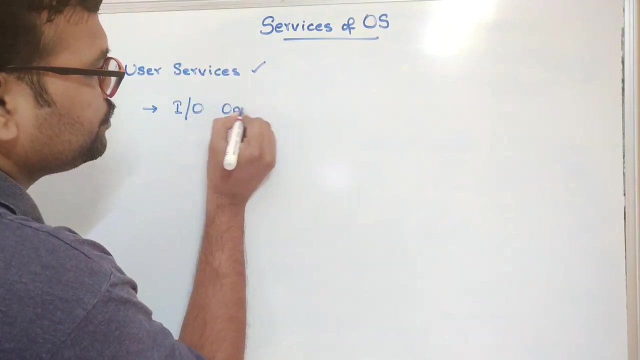 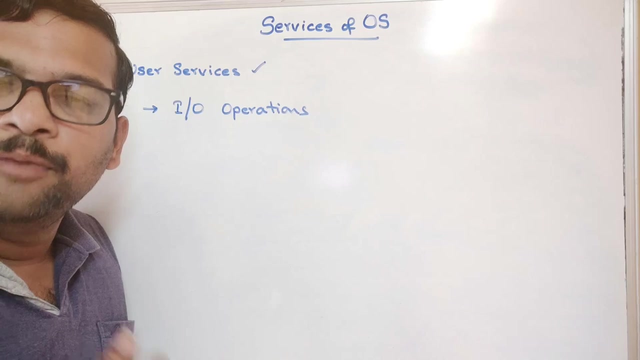 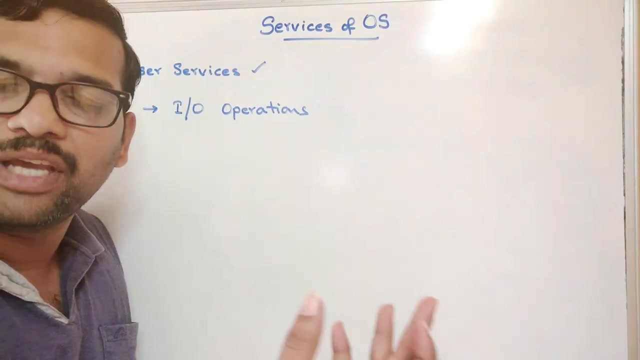 services, so two, and the third one, Ivo operations. so coming to this third service, so we know the Ivo devices: input devices and output devices. so thus the user will use the input devices to give the input from, to give the input to the system, and the system will give the output by using 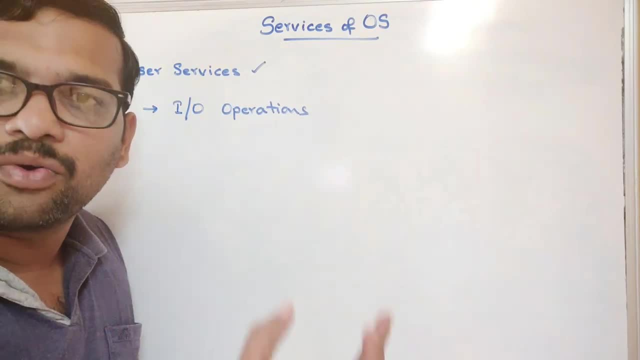 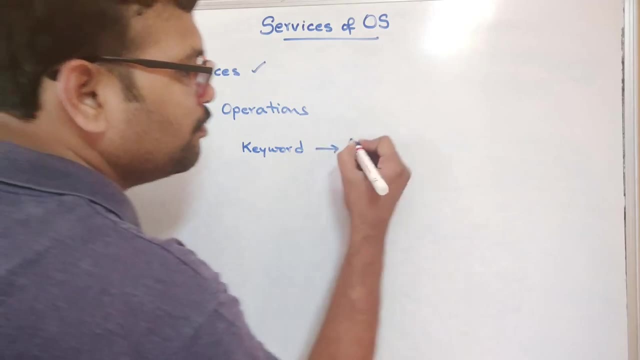 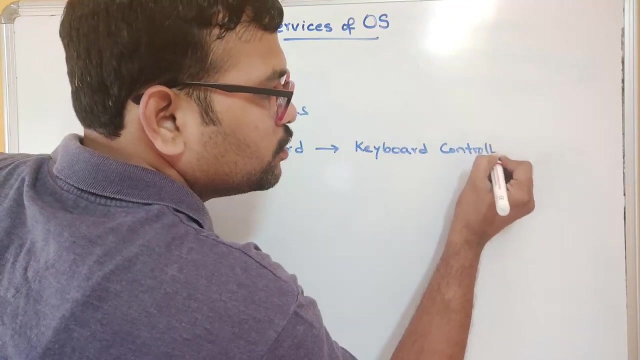 the output devices. for every Ivo device there will be a controller, right. so, for example, if you are using some keyboard to give the input right, it is having some keyboard controller, keyboard controller through which we can communicate, right. so next, if you are using some memory, there will be some. 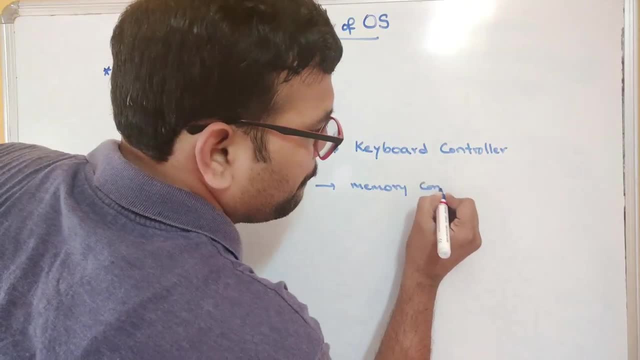 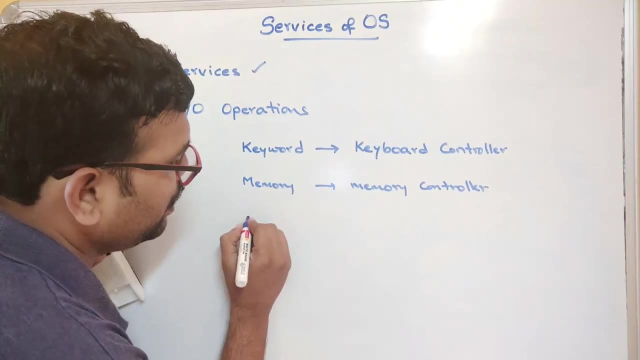 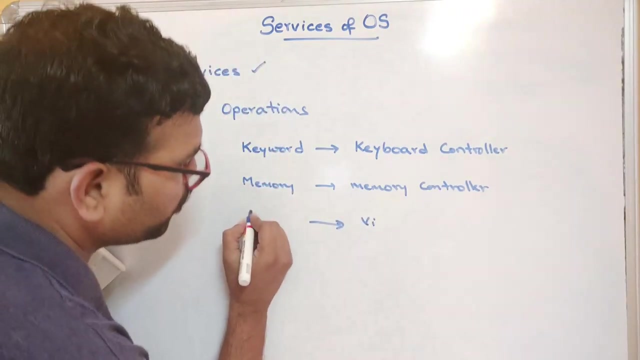 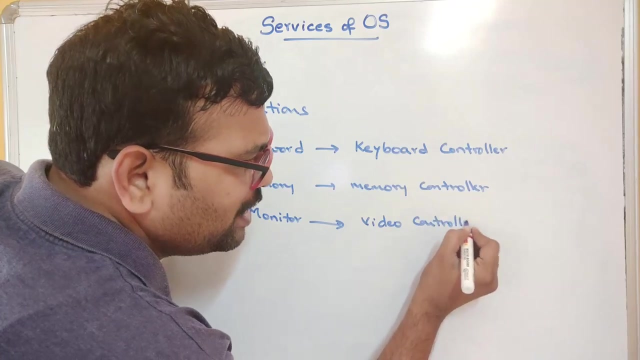 memory controller and if you are using any video, so we will be having so. if you are displaying the output on the monitor- example, right, this is the best example- so we will be having some video controller like this for all the Ivo devices will be having a different controllers and through this video can't. 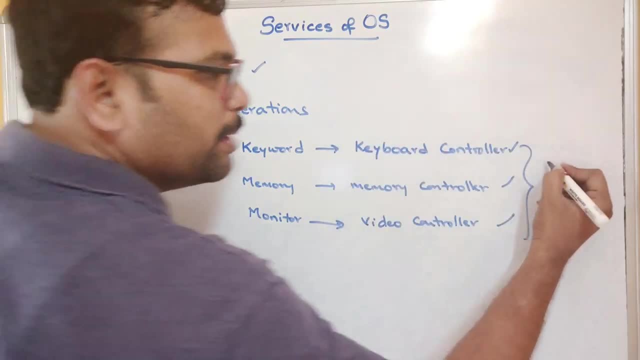 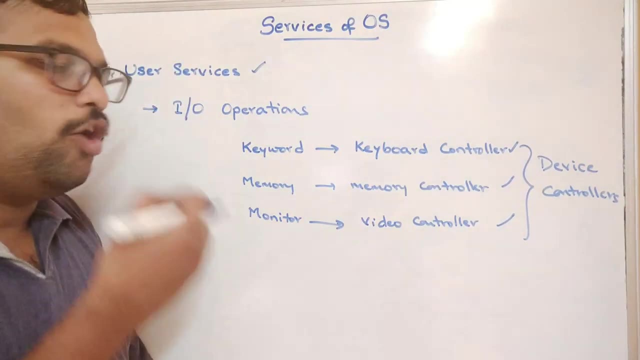 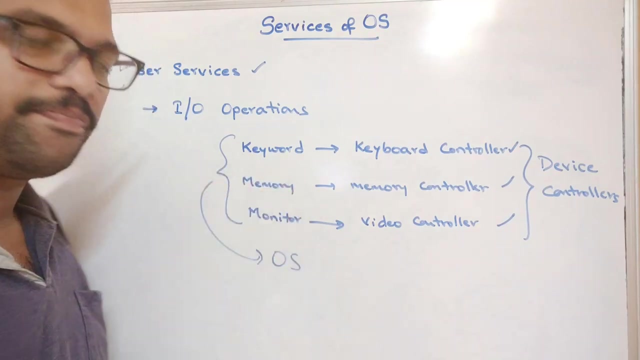 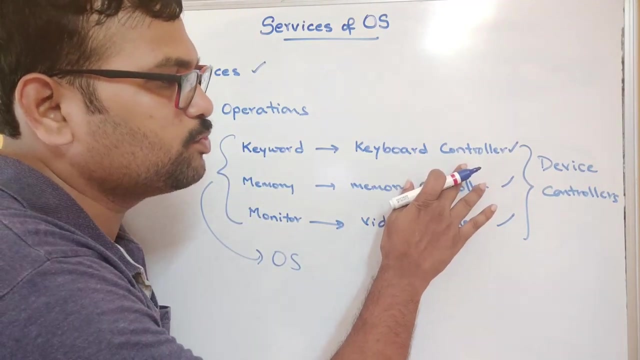 we will come on the use the device controller. we will commonly call them as a device controllers. okay, device controller. so by using these device controllers, so the operations will be communicated and all these controllers will be maintained by the operating system. okay, so these Ivo operations will be executed smoothly with the help of these controllers which have maintained. 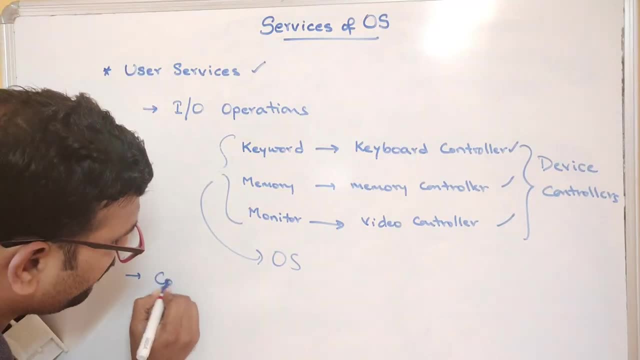 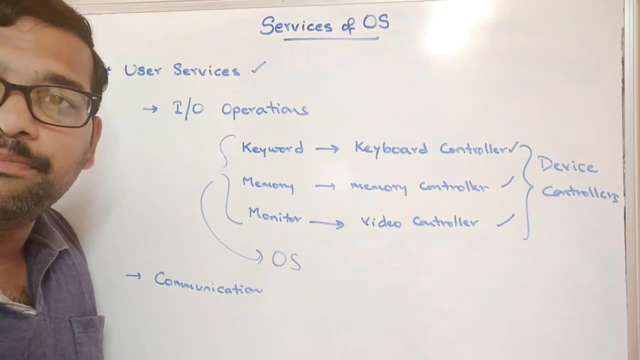 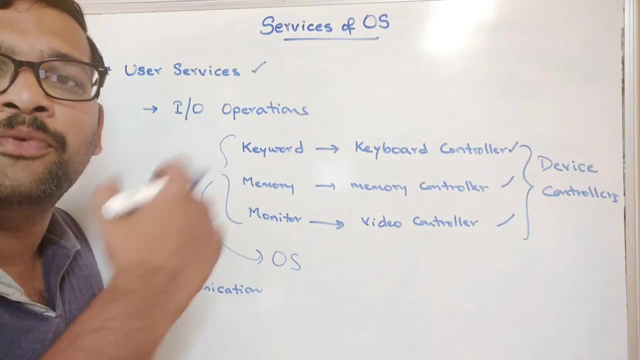 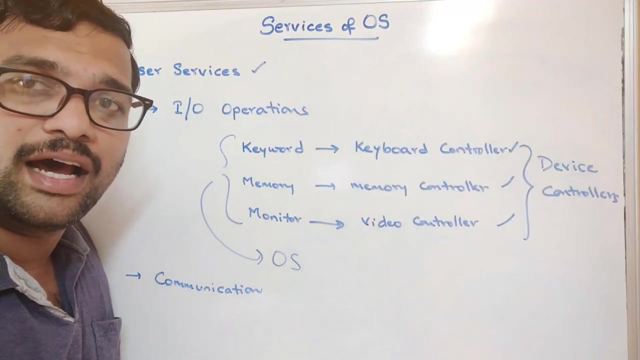 operating system and the next one communication. so here the communication means. so in our system there will be a lot of processors executing right, so if one process want to communicate with another process which may reside in the same system or another system, so if we call it is and the 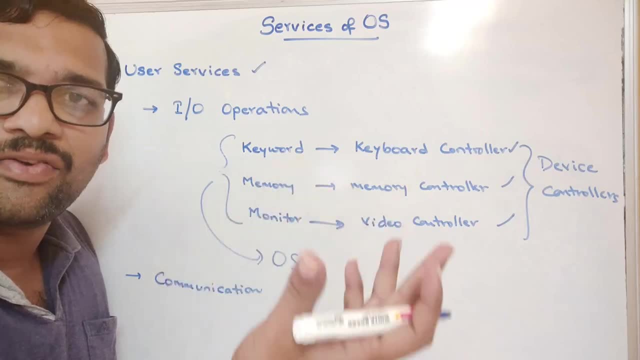 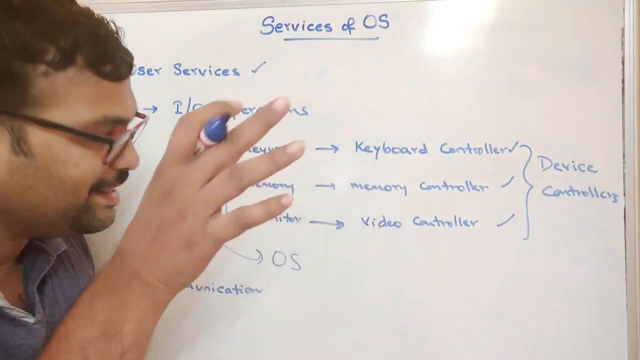 another system. we call it as a network, right, if two systems are in a network, so there should be some sort of communication right there. some sort of communication should be done between the processes, and that process will be maintained by this communication, and this is also a service. 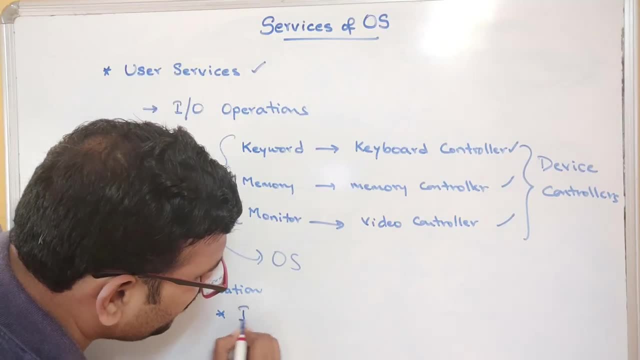 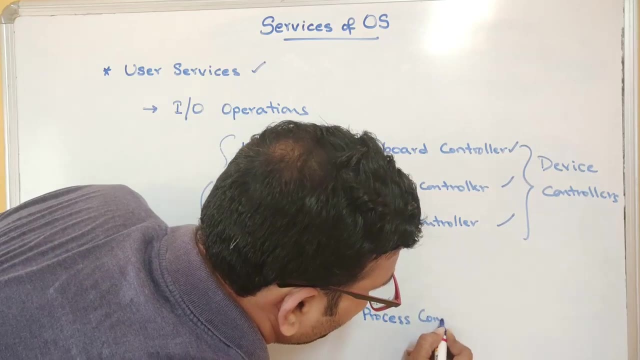 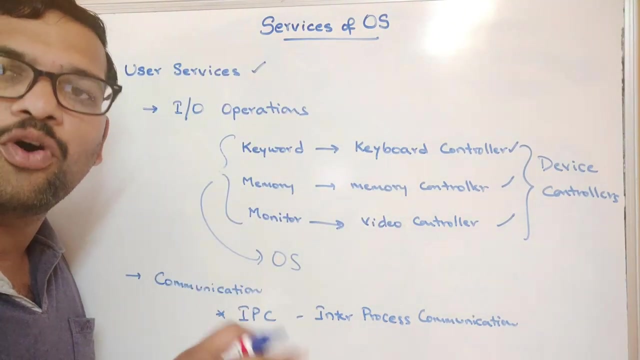 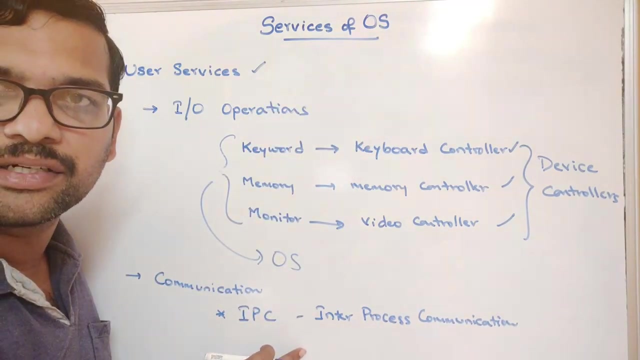 provided by the operating system, and this we call it as IPC is inter process communication. inter process communication, so in order to communicate between different processes which are maintained in the same system or in different systems, so this will be used. i mean, the operating system will take care about this communication. 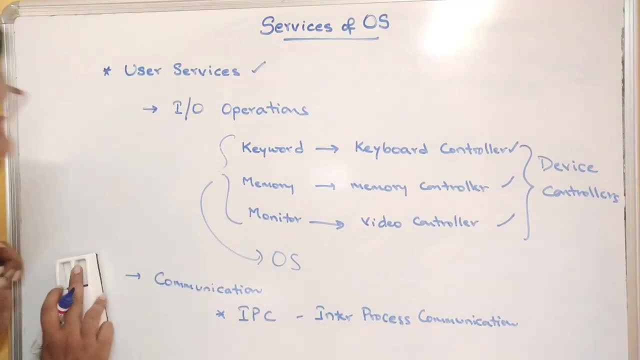 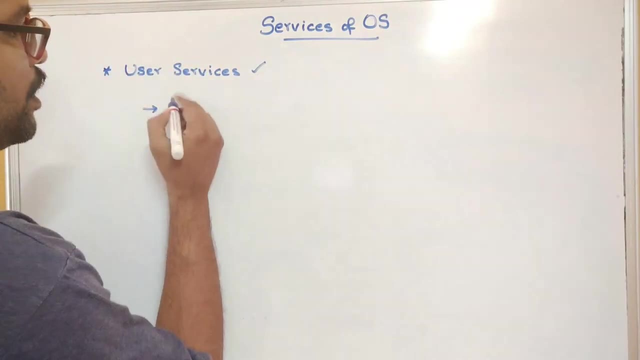 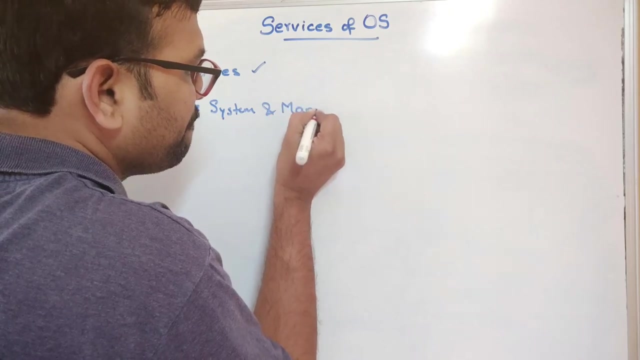 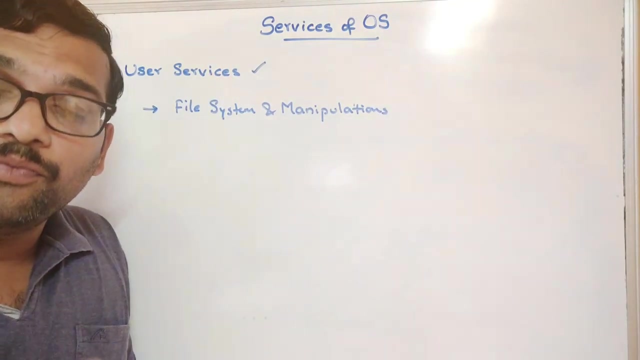 right between different processes, then the next one, the next one, file system, file system and manipulations. so coming to the file system, so the we, we are going to write the some data onto the files. we can read the data from the files and we can store the. 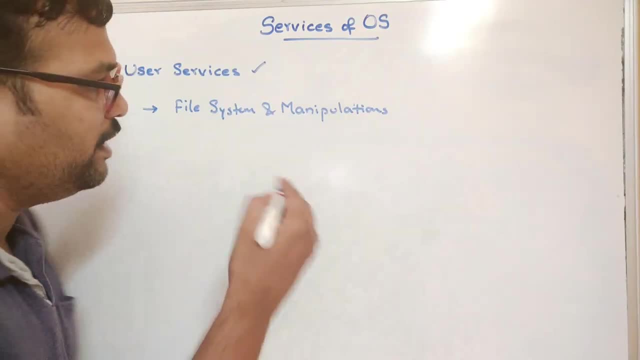 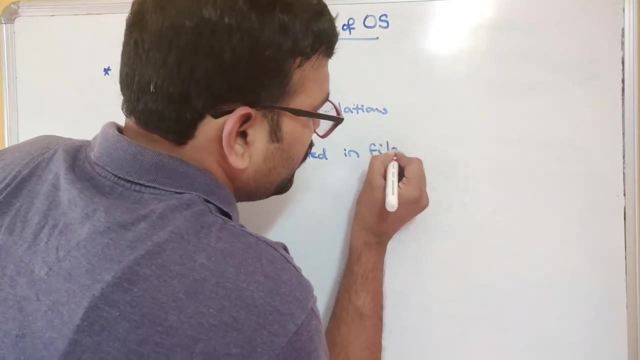 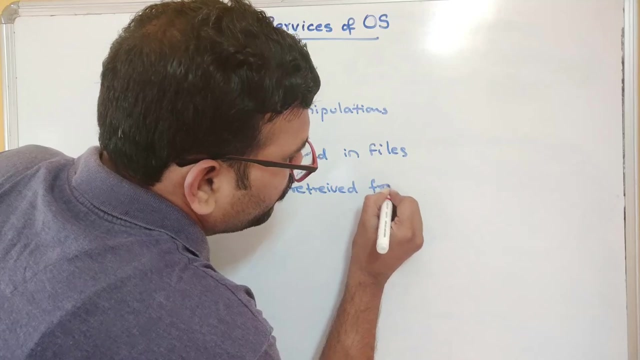 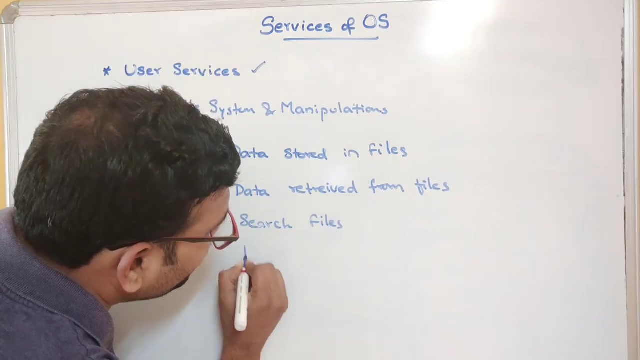 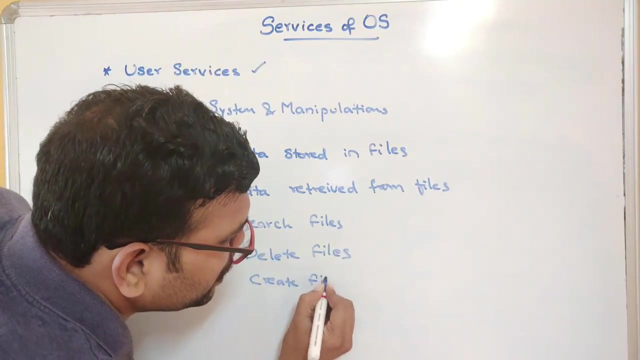 files in the memory. so everything will be done. right, the data. the data can be stored in a files. right, and data can be retrieved from files and we can search the files. you can search the files and we can delete the files. delete the files and also we can create the files, we can create the finds. so 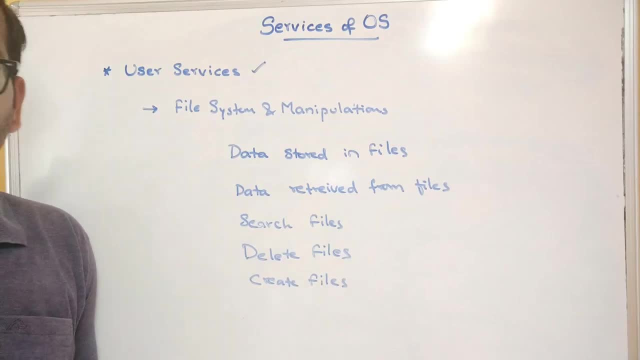 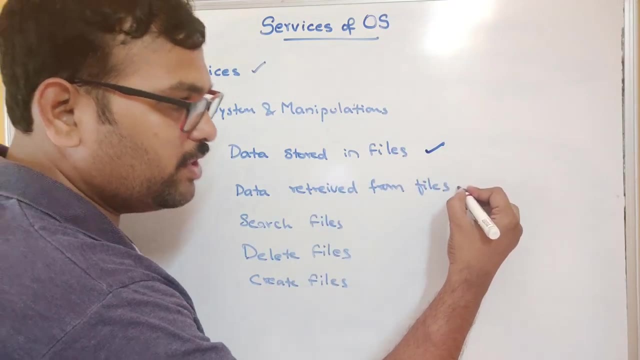 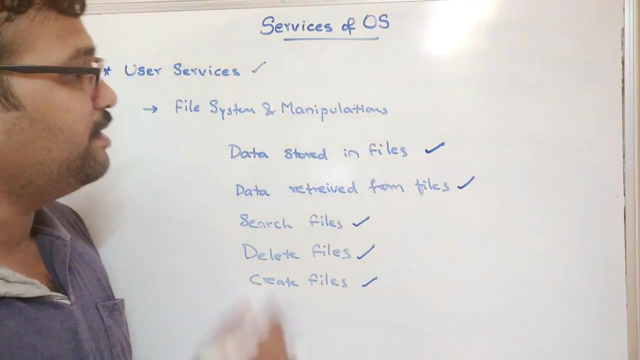 you will be having the data right, so the file will be having the data and we are going to search the file. we can store the data into files. we can retrieve the data from the files and we can search the files. we can delete the files, we can create the files. so everything will be done with. 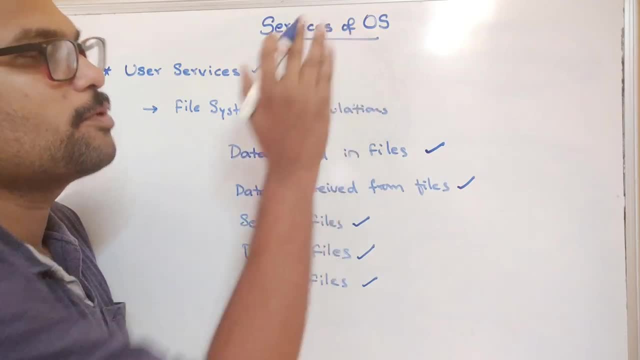 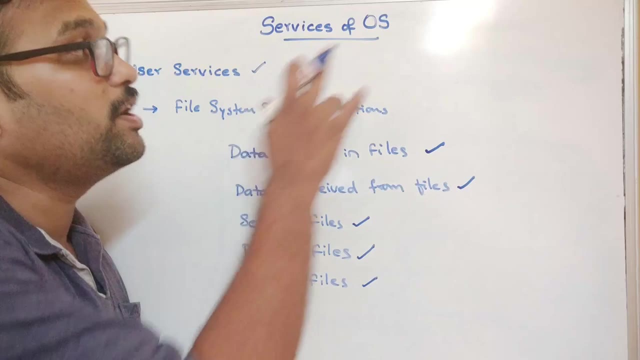 the help of this finding system and manipulations, which is the service provided by the operating operating system, So we can do these processes in this service, and this is a service provided by the operating system. So without operating system it would be very difficult to search. 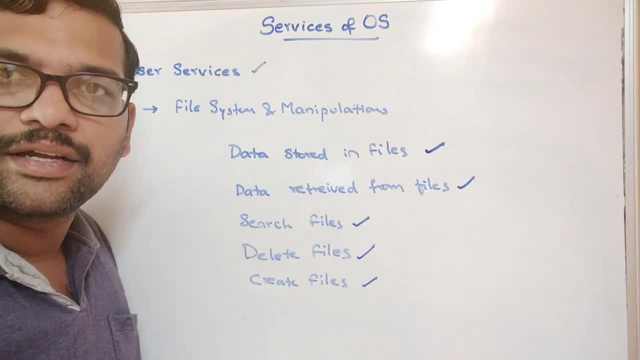 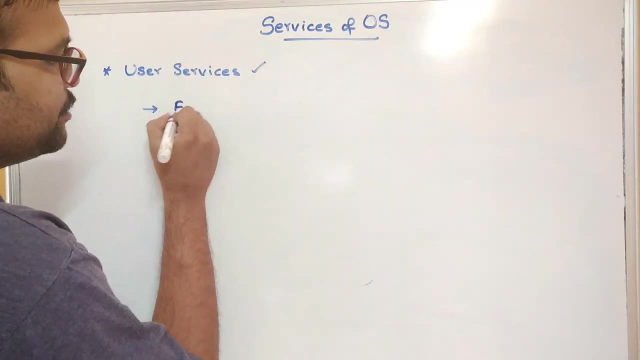 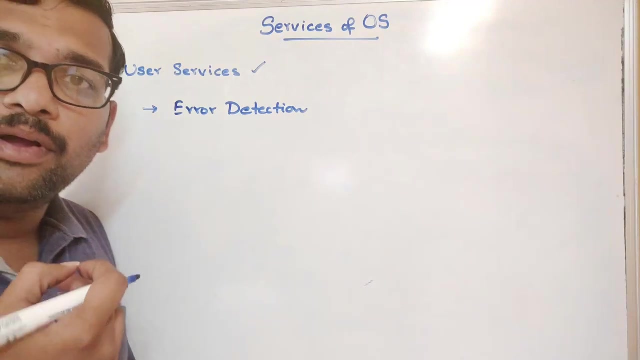 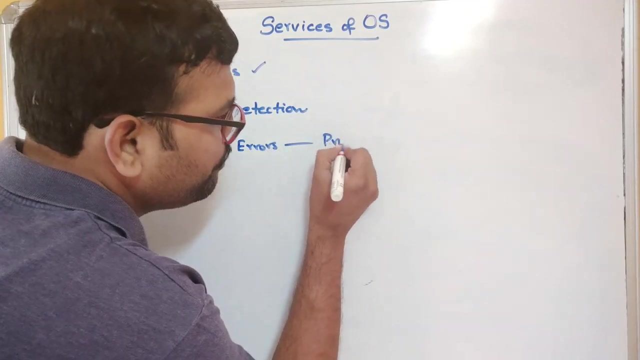 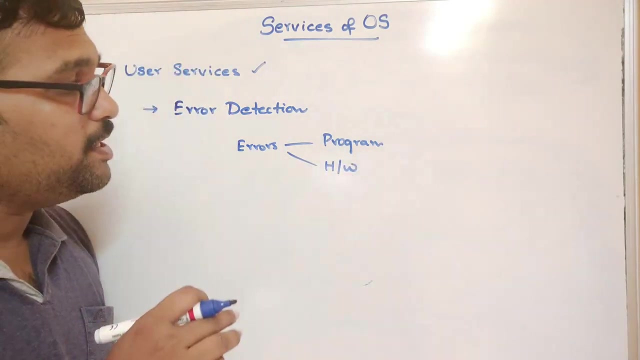 the files. or we can manipulate the files, or we can create the files right. And the next one, error detection. error detection: So while executing the program some sort of errors may occur. So errors may occur in program or in hardware, right, So the operating. 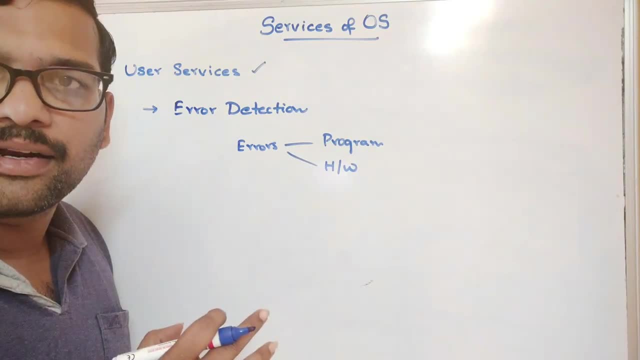 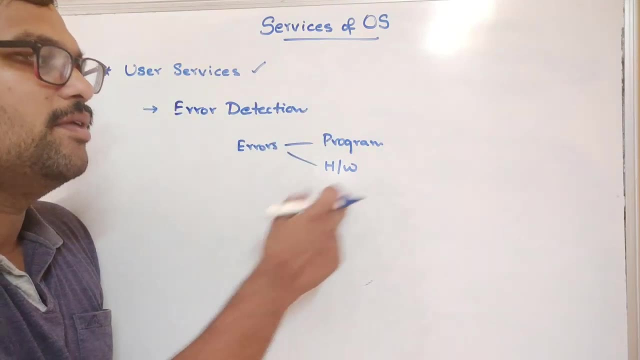 system should know about all the errors that may occur, right? So this, the service provided by the operating system, is these errors, which are occurred from the program or the hardware, should be reported to the users. So errors, so, whatever the errors are, they should be. 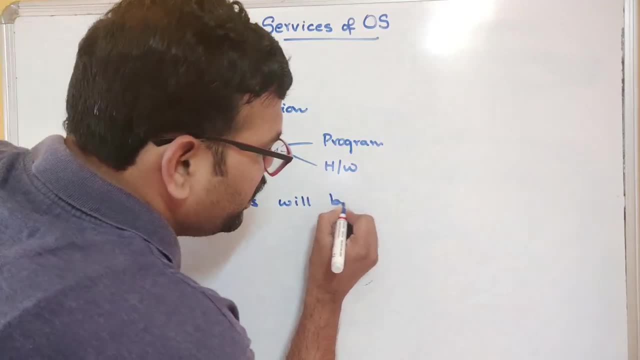 reported to the users. So errors, so whatever the errors are, they should be reported to the users. So errors, so whatever the errors are, they should be reported to the users. So errors, so whatever the errors we are getting, those errors will be reported to. 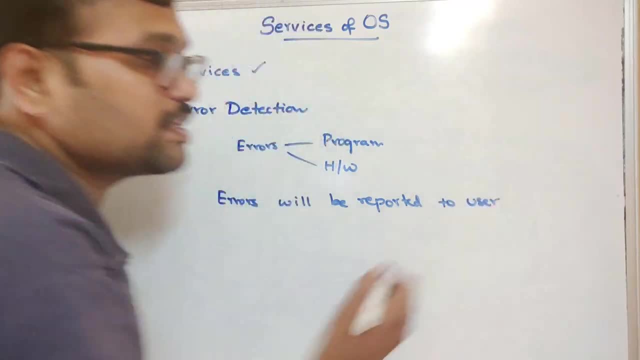 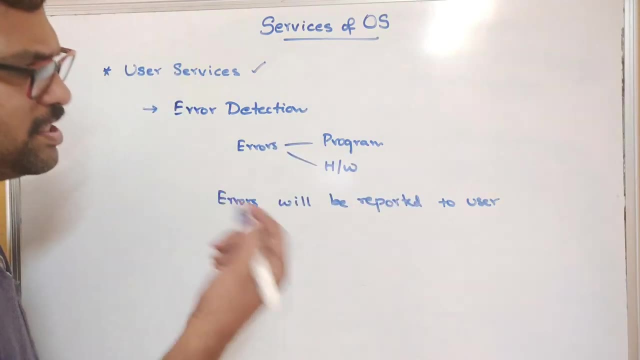 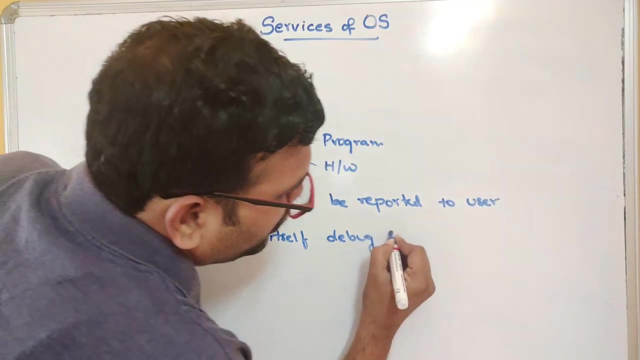 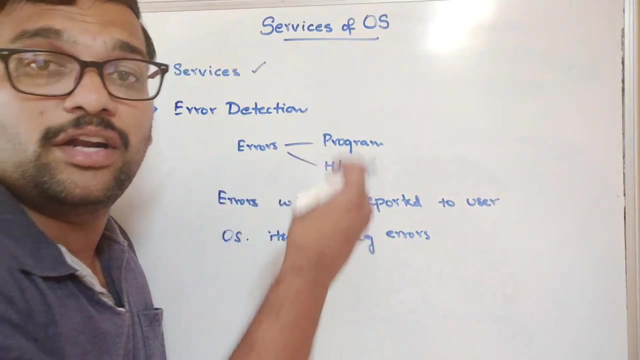 the users So that the users can take a certain operation to debug those errors, right? So sometimes the OS itself has the OS itself debug the errors, debugs the errors. So if the errors occurs, so OS itself debugs the errors, otherwise the errors will be reported. 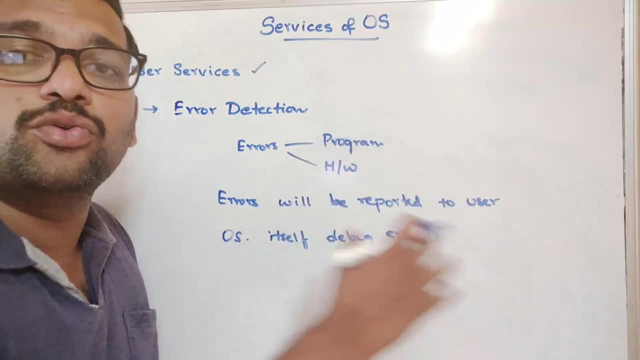 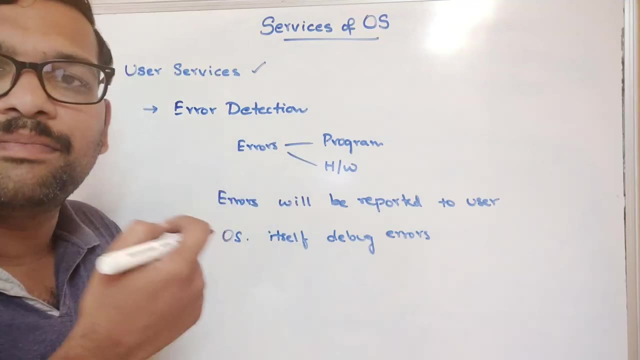 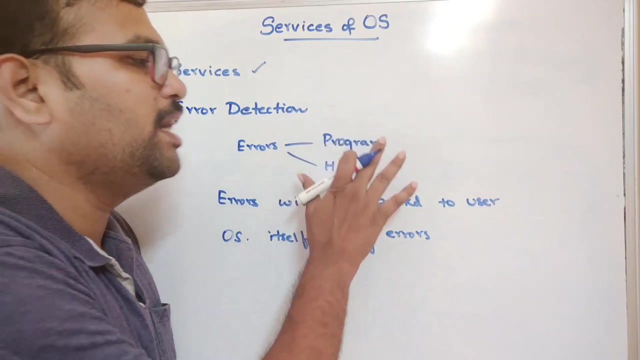 the user so that user can take appropriate action to resolve those errors. so this will be maintained by the operating system and by using this one, the system can work consistently without any errors. without any errors. okay, the errors can be occurred from either program or any hardware, hardware. 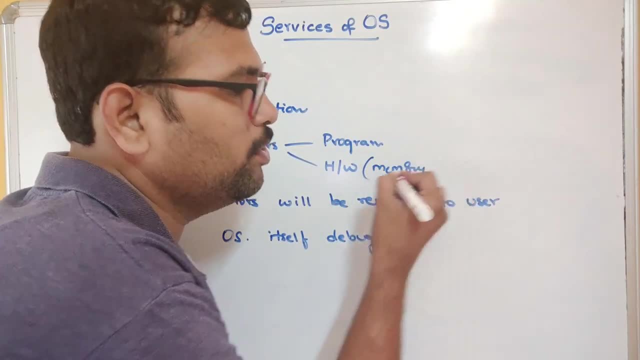 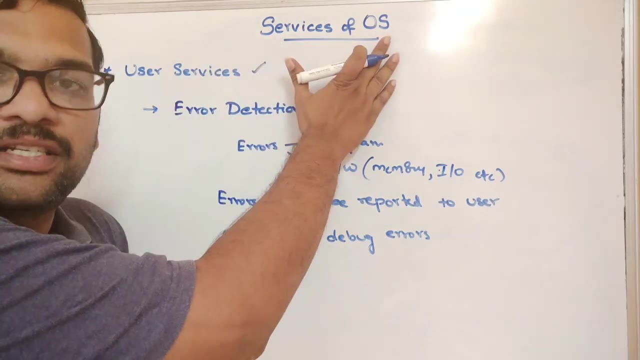 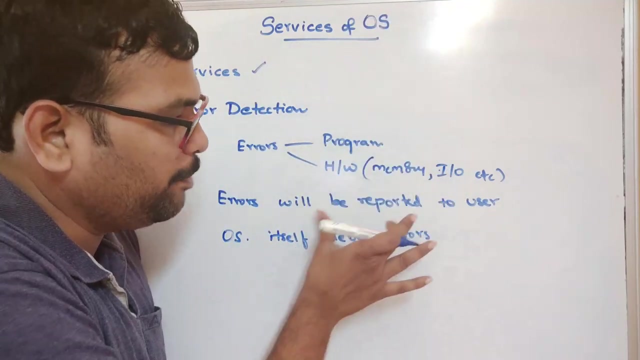 it seems like, from the memory point of view, or some ivo point of view, etc. so, whatever it may be, everything should be known by the operating system. so all the errors that may occur must be known by the operating system, right? and those errors should be reported, or some. 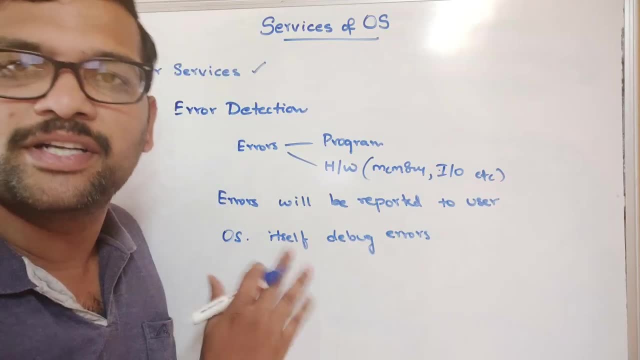 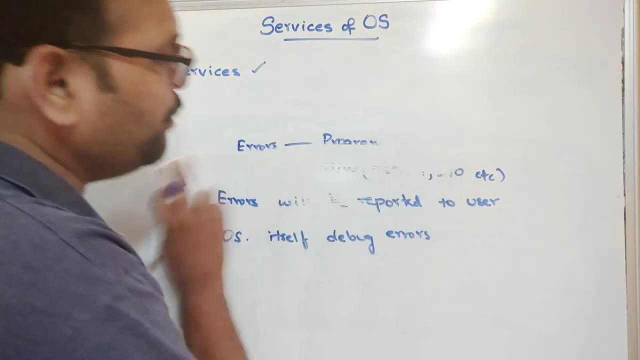 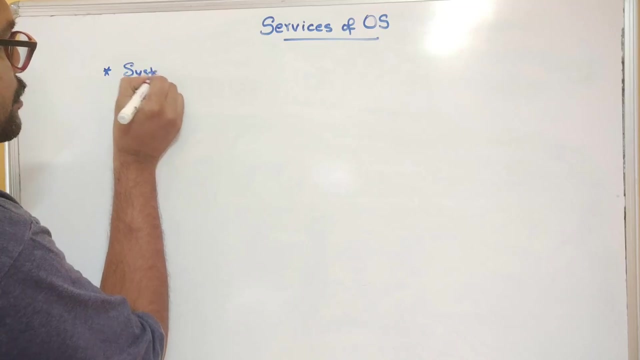 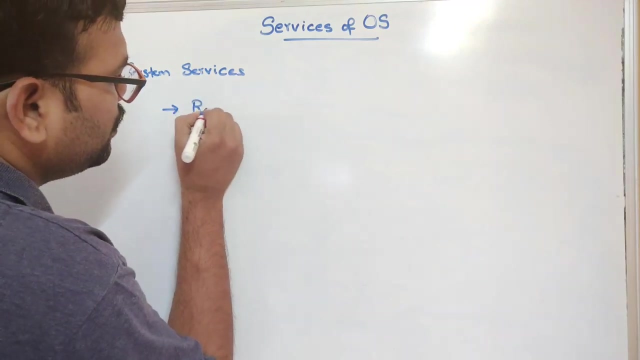 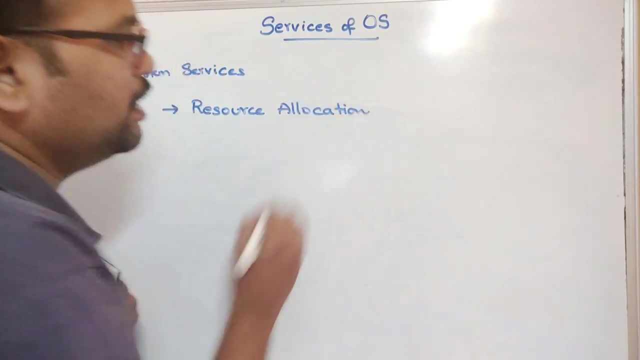 some sort of errors can be debugged itself. the operating system will take care about that one, right? so these are all called as a user services, right? and then coming to the system services. so there are a few services, system services. okay, so the first one is resource allocation. resource allocation so that means if a program or a process 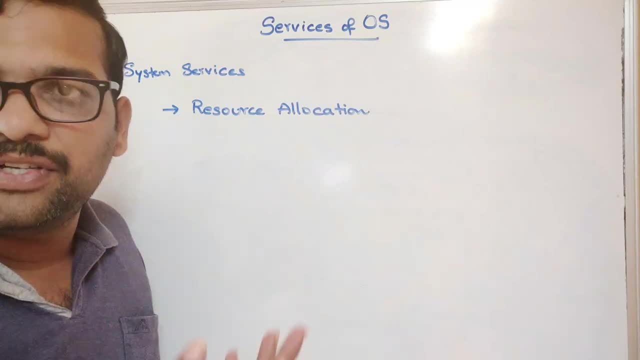 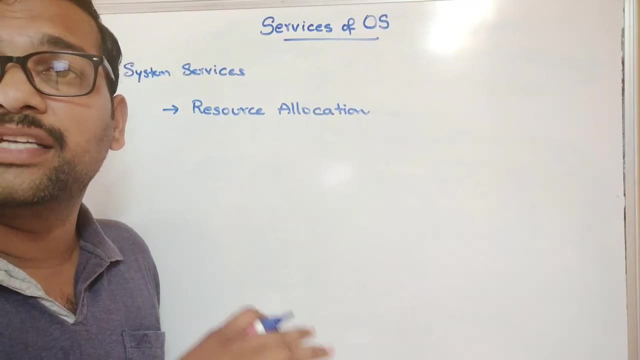 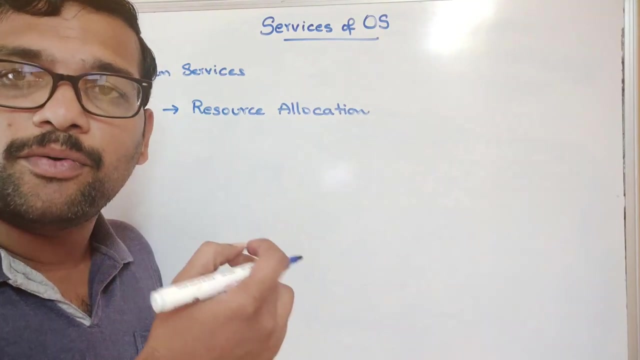 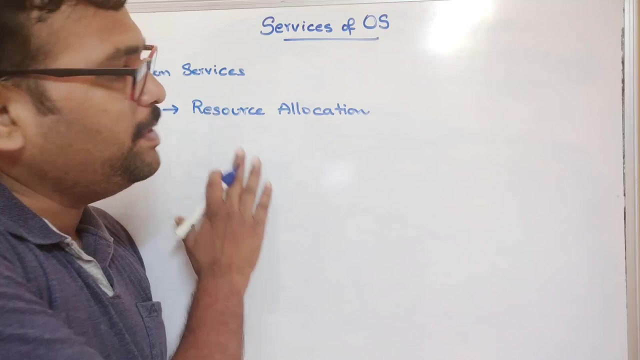 is being executed, so it may require a lot of resources. so, similarly, our operating system can- uh, i mean more than one process can be executed at a time, and multiple resources should be allocated to different processes, and sometimes one different process may require the same resource. okay, all these ways, so the resource can be allocated to each and every process. 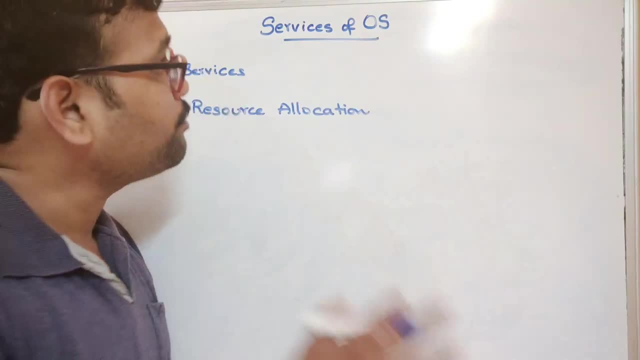 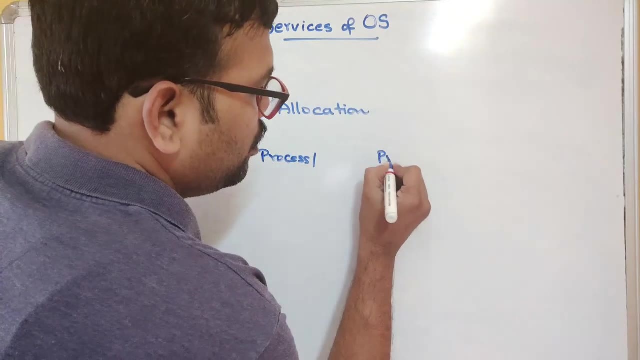 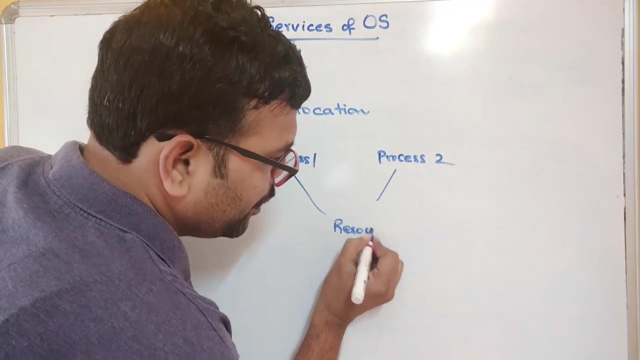 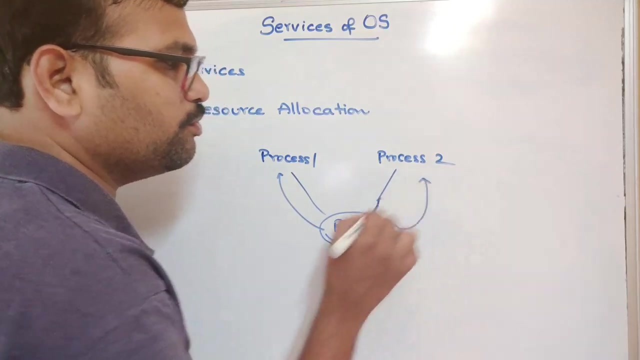 without any overlapping right. so that process will be done by the operating system. so we can have a different processes: process one, process two. so if both are using the same resource, so without much waiting time, this resource will be allocated to process one as well as process two, with a less waiting time, because if the process one is using this resource, this process two. 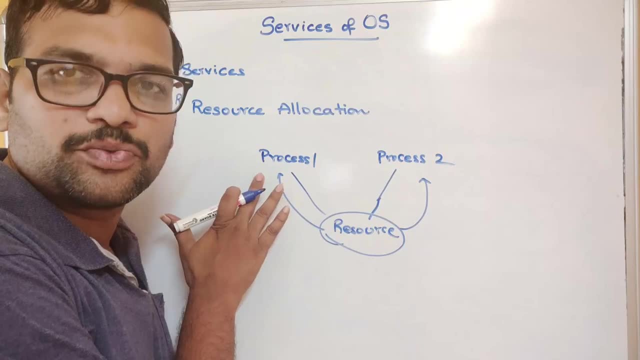 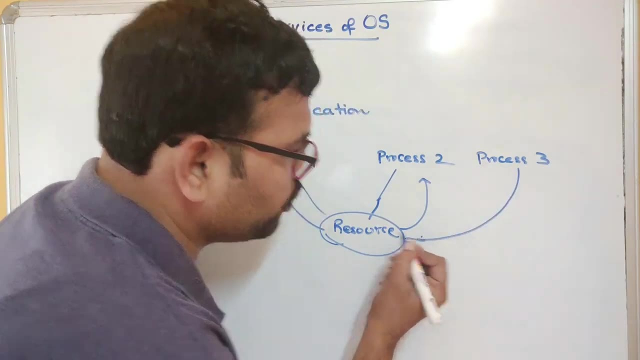 has to wait until this resource is released by the process one. so if there is another process, process three, and if it is also using the same resource, so then this process three has to wait until the resource. and then I will now talk about process, about the process one and process two. 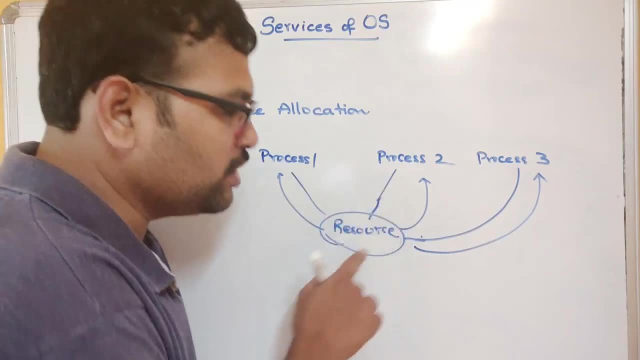 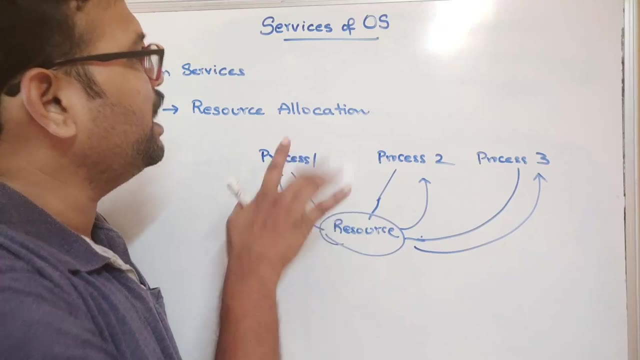 process as well. reason: 해� corporations stay tuned until hevideozeedling team being released by process 1 and process 2. so this resource allocation, resource allocation with a less minimum, that means a minimum waiting time- the resource will be allocated by this operating 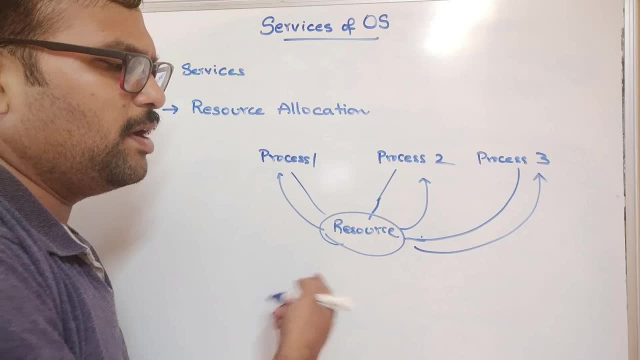 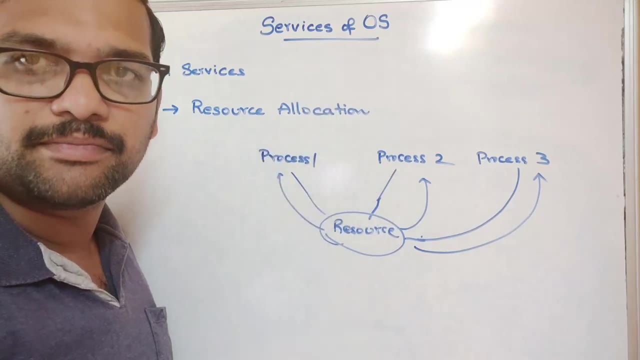 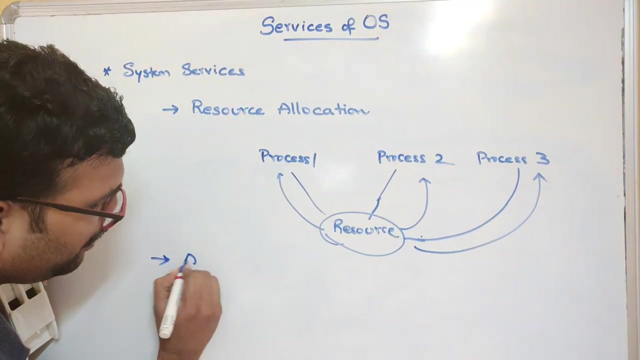 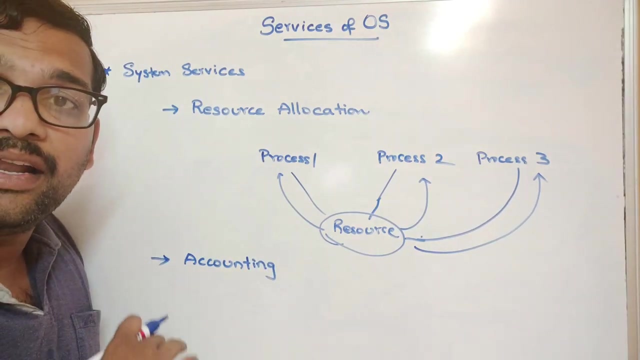 system and similarly different processes can access a different resources. so optimal utilization of resources can be done by the operating system. okay, so this one is a one service and the next one is accounting. so accounting means operating system will provide a different accounts for different users. okay, so multiple users can have a different accounts so that every, each and every. 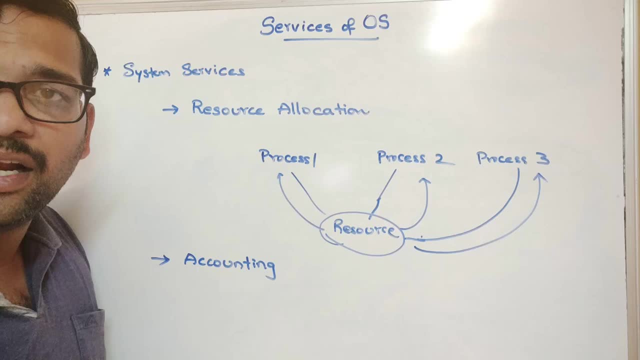 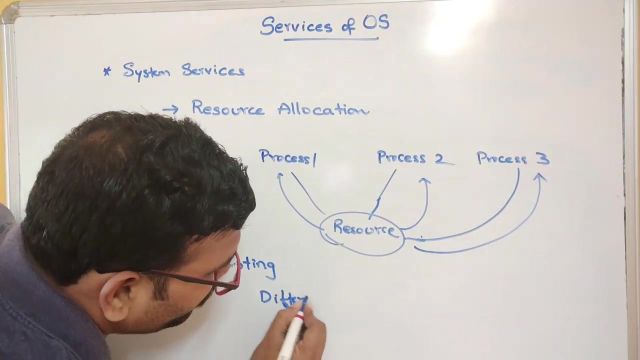 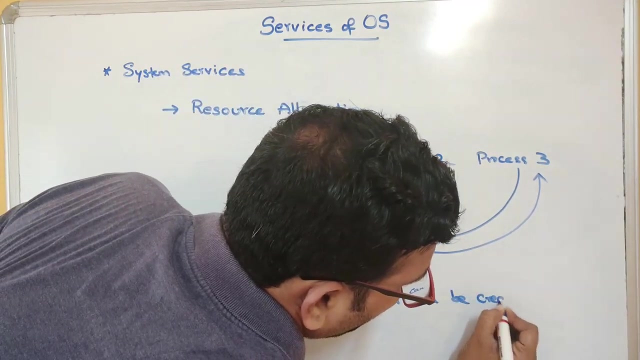 user will be having a different operations right. so all the log of particular user can be maintained by the administrator. so what actually is being done by individual users will be maintained by the user administrator right. so different accounts, different accounts can be created for multiple users, for multiple. 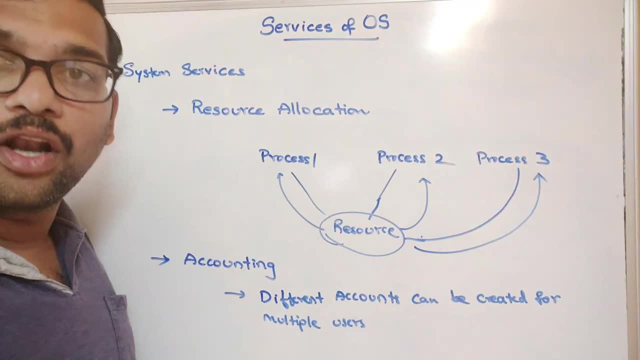 users. so every log- okay, the log of user. log of user means whatever the operations being done by the user will be maintained in a log and all these logs will be keyed in a log. and all these logs will be keyed in a log and all these logs will be. 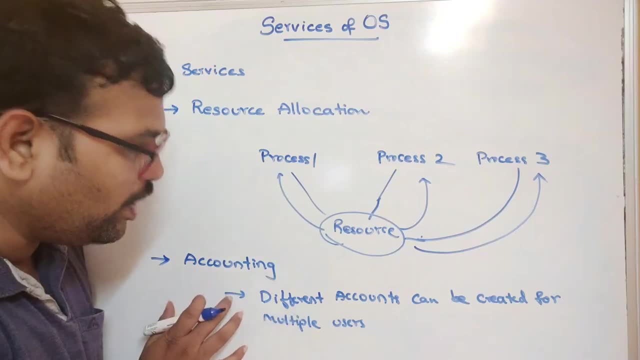 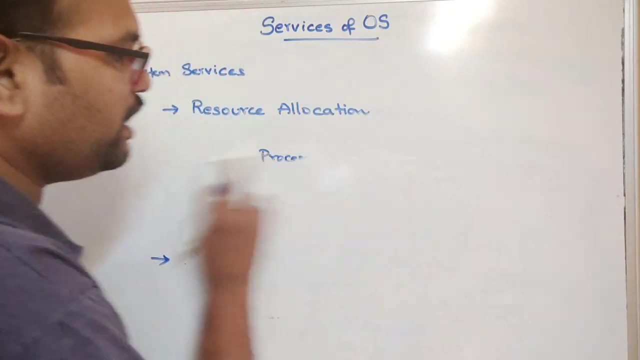 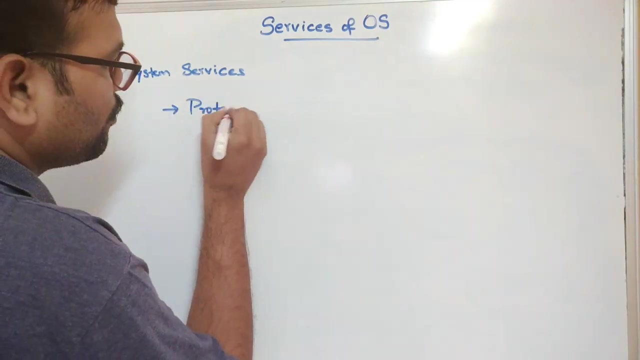 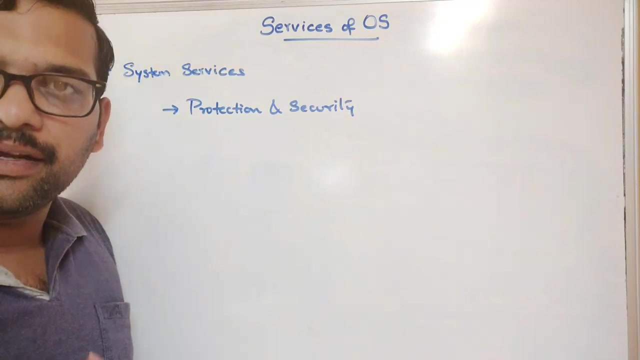 keep on monitoring by the administrator right. so this is one service provided by the operating system and the next one is security and protection. it's also very important, security and protection, so we need to provide the security for the data. okay, we need to provide the protection and 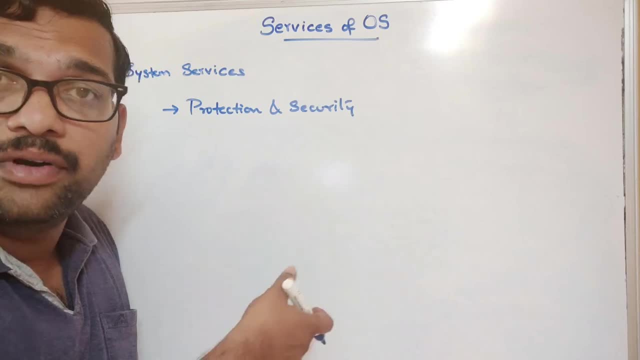 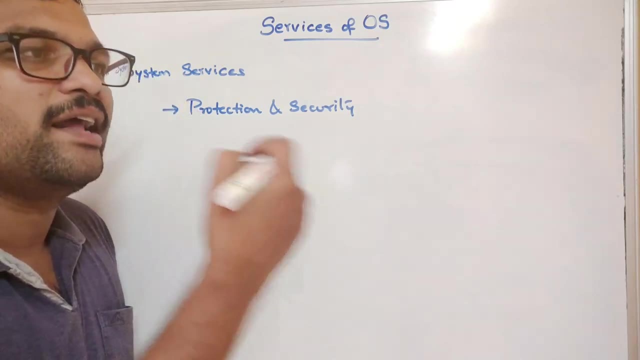 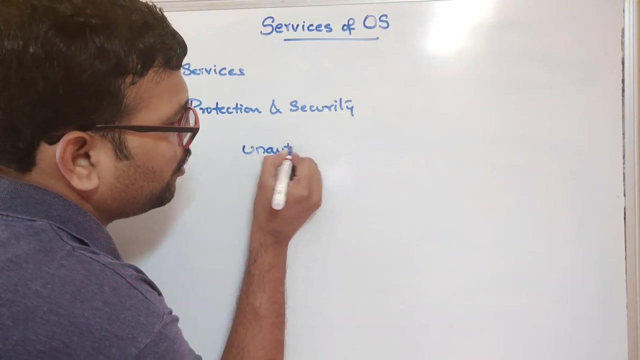 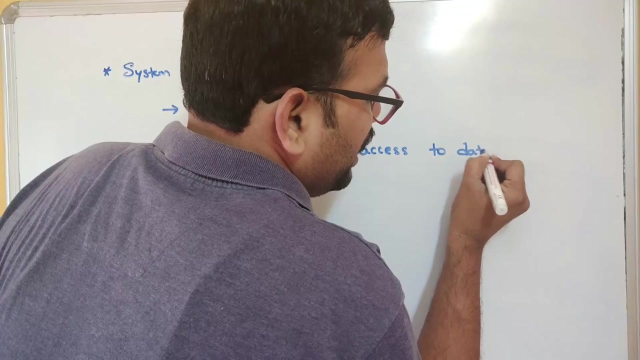 security for the data. so in the previous service, that is, our accounting, we are providing- i mean the operating system is providing different accounts for different users so that one user can't access the data of another user. okay, so we can prevent from unauthorized access, unauthorized access to data and files, and also we'll use some. 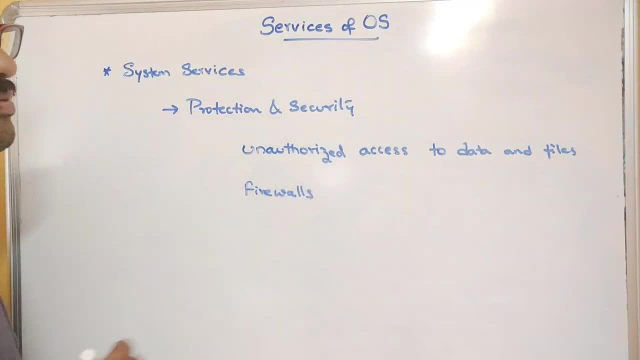 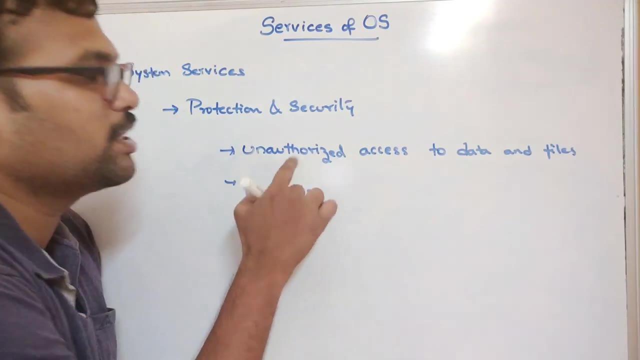 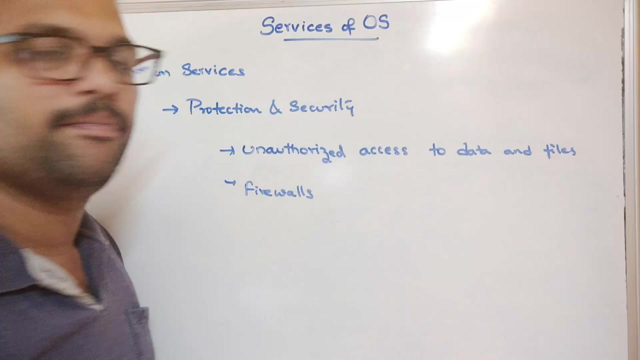 firewalls. firewalls, okay, for the security purpose. for the security purposes, all right, that security purpose. okay, we'll use some firewalls and we'll use some unauthorized access. okay, we'll have the. we'll protect the data from unauthorized access to the data and files, because 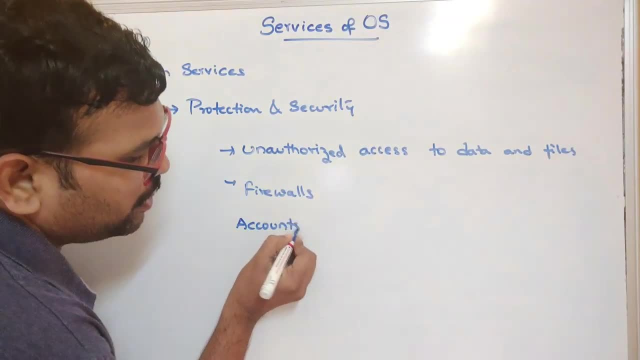 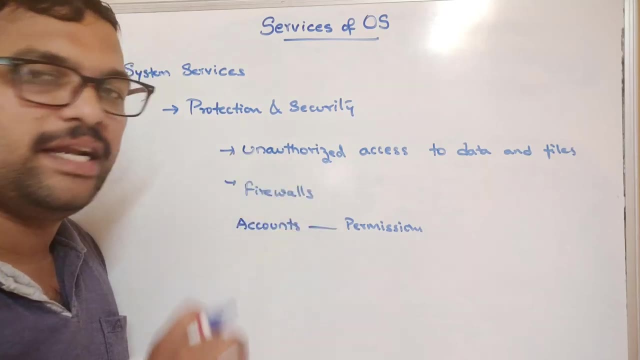 accounts will be having a permissions- okay, accounts will be having some permissions- permissions. so, based upon the permissions, only the users can access the data who have the permissions. okay, so without the permission, the data cannot be accessed by the unauthorized persons. so by this, the protection and security will be achieved, and this is also one service provided by the.